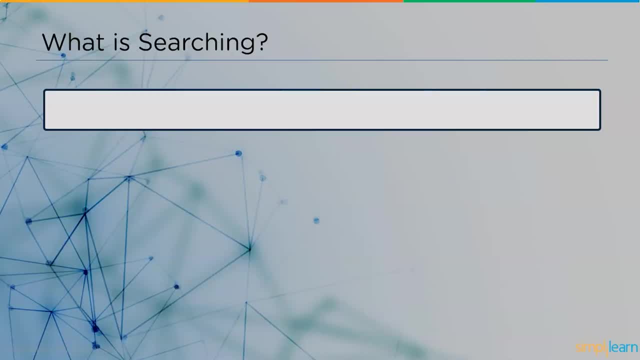 searching can be categorized into two types. First type is the sequential search in which we check the elements in a data list or an array, one by one, In data structures. searching can be categorized into two ways. The first type is a sequential search in which we check the elements. 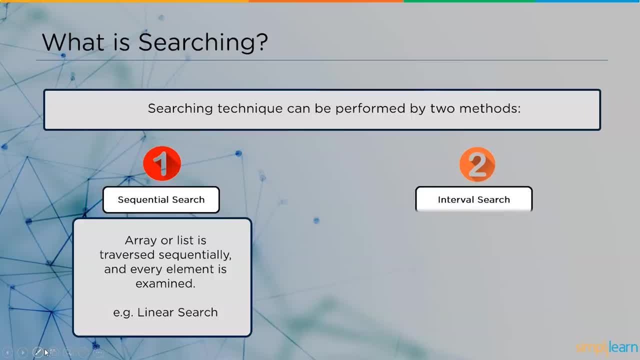 in a data list or an array, one by one. An example for sequential search is linear search. Now let us learn about the next type of searching approach. The next type of searching approach is the interval search approach. Interval search divides the search in half by repeatedly targeting. 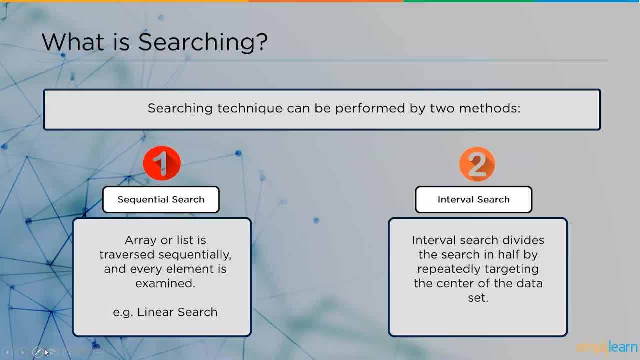 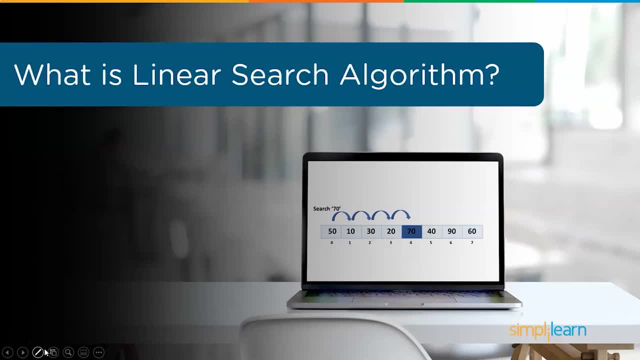 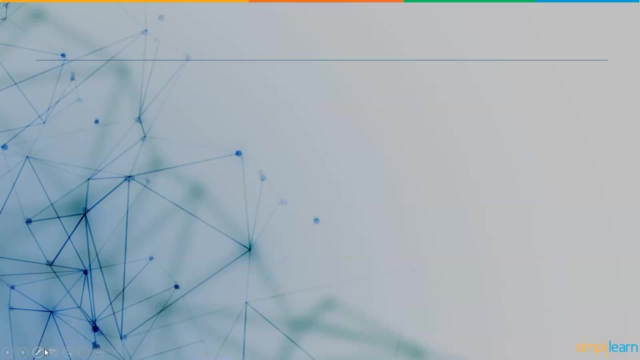 the center of the data set. The binary search algorithm can be an example for interval search. We will go over the binary search algorithm in detail in our upcoming video. After understanding the logic of search and the types of search, we will get into understanding what is linear search algorithm. 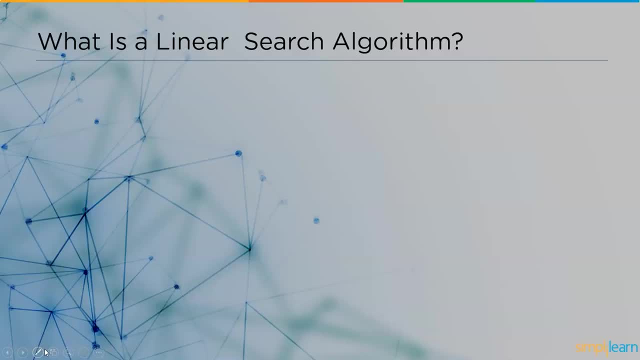 The linear search method is a simple search technique. In this type of searching approach we perform a sequential search across all objects, one after the other. Every element is examined and if there is a match found, then the specific element is returned. Otherwise, the search 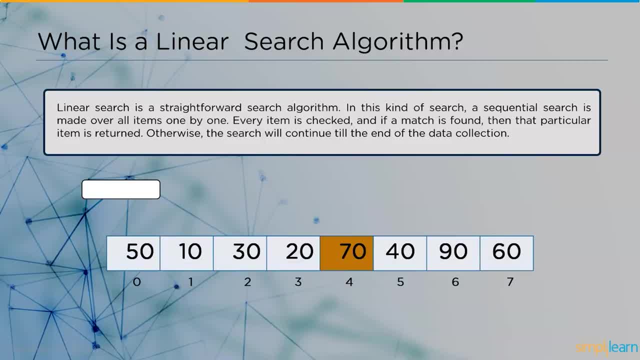 will continue until the data gathering is complete. Let us go through an example for better learning experience. On my screen we have the following elements: 50, 10, 20, 30, 70, 40, 90, 60 as randomly distributed elements. Let us imagine that our target element is 90.. 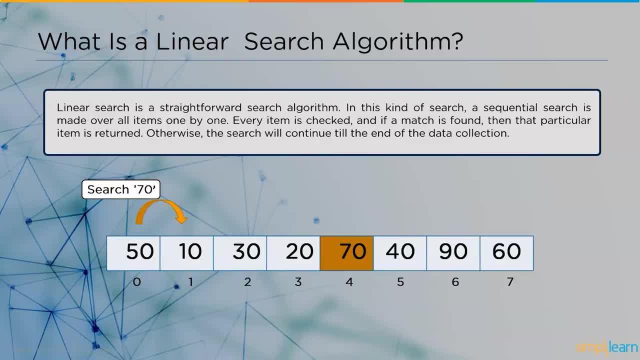 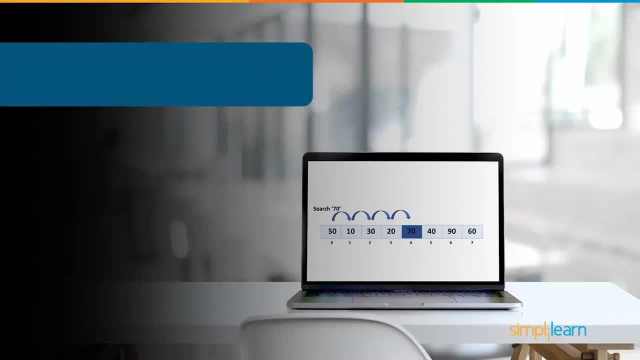 We found that our target element was 70 using linear search strategy. So how does it work? In the next segment we will look into the working terms of linear search algorithm. The simplest method of searching the data collection is linear search, Starting from. 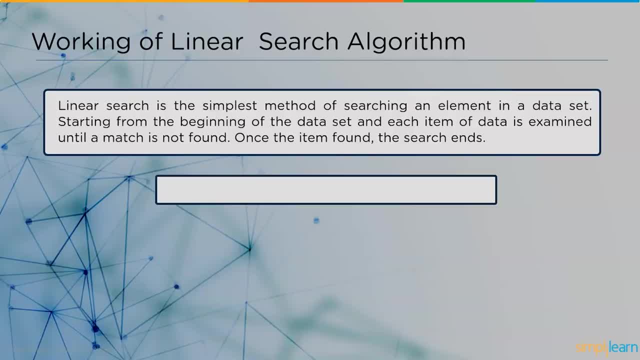 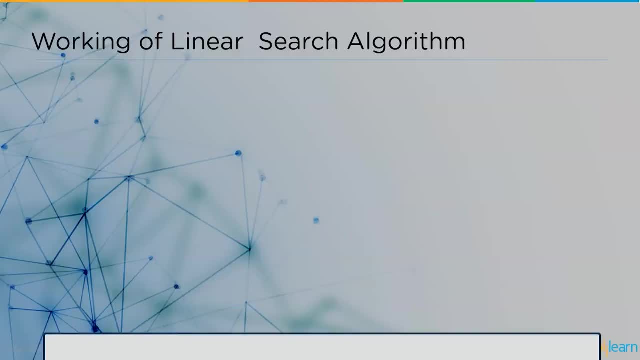 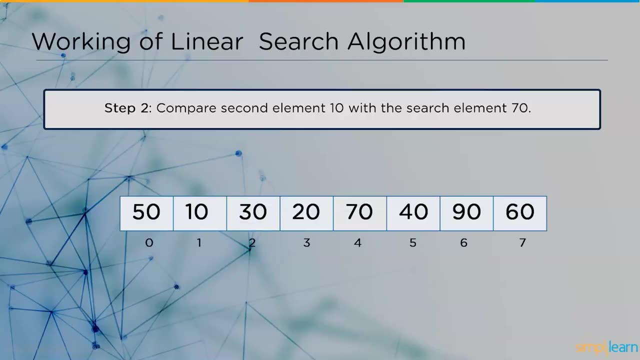 the beginning of the data set. each element is examined until no match is found. The linear search completed after the item has located In the first stage. we compare the first element, that is 50, to the searched element, that is 70. We will go on to the next element, because 50 and 70 are not matched. 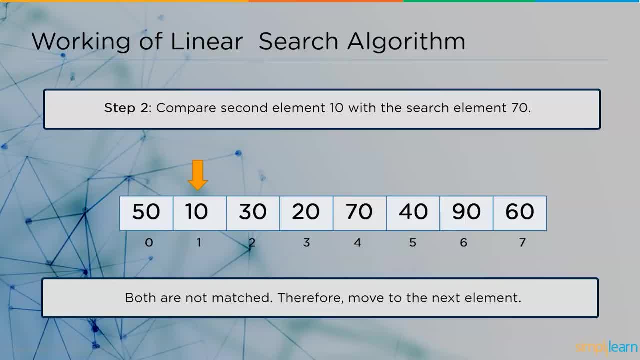 We will compare the second element, which is 10, to the search element, that is 70, in the next step, And once more there is no match found. Then we have the element 30 as the next comparison, and 70 and 30 are not matched. 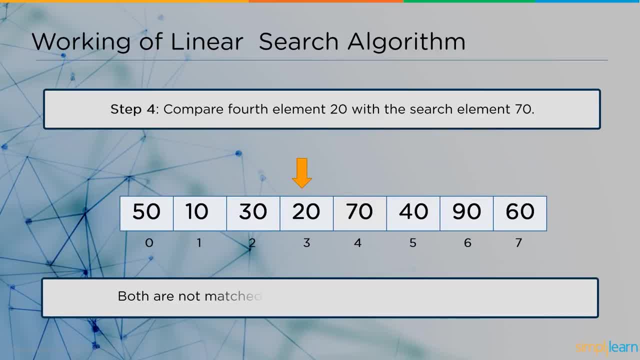 We have the next element, that is, 20, in the fourth phase, and there is no match when we compare 20 with 70.. Moving on to the following stage, we have the data element 70 and after comparing 70 with the search element, there is a match. 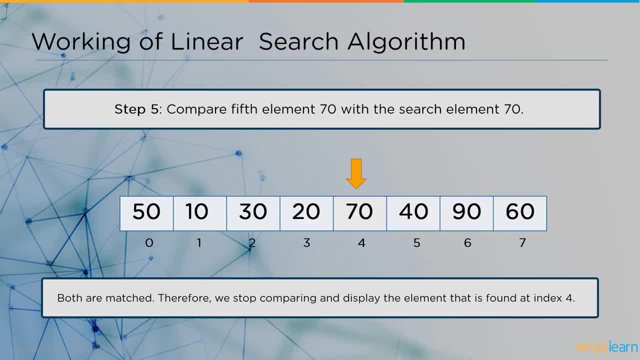 We will now have the searching and display index as 4, and this index contains the searched element. We now comprehend the search. We will now have the search and display index as 4, and this index contains the searched element. We will now understand the pseudocode of the linear search algorithm after learning. 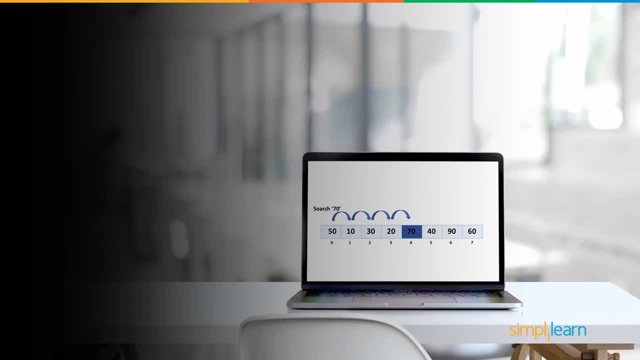 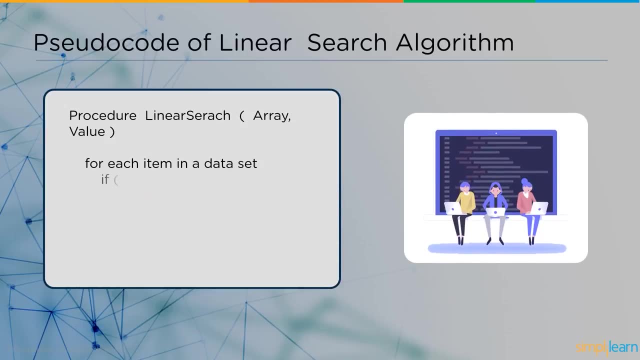 the working terminology of linear search algorithm. First, we have a function called LinearSearch which has two variables in its parameters: The ArraysName, which is an array, and the searchVariable, which is the value. Then, using a for loop, we must search for our target variable by analysing all the data. 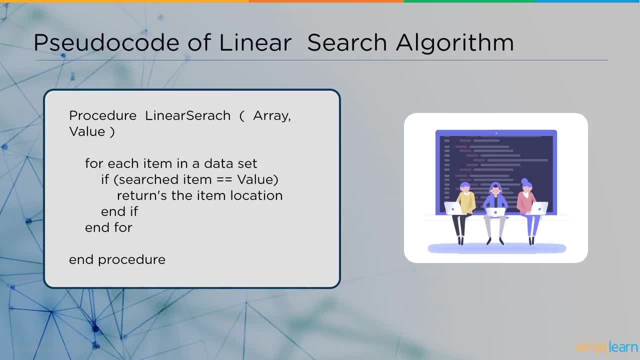 elements in the dataset. with the condition, that is, the search item is identical to any sets value, we must return its index value Now. we must stop searching once the searched value has been discovered. Then we will close our if and for loop, as well as the linear search function. 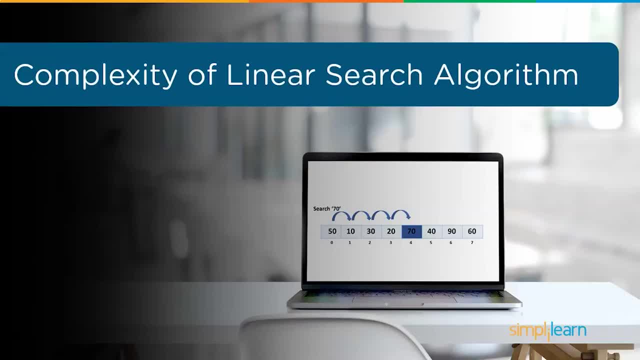 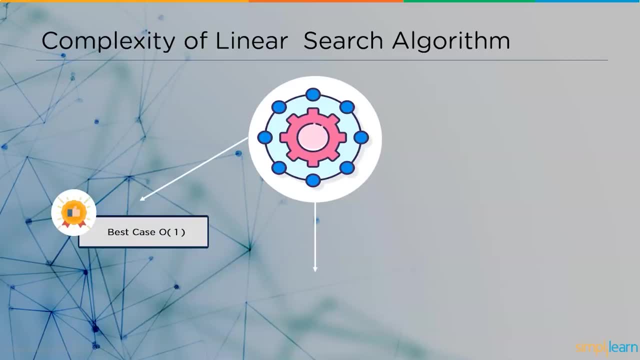 We will now look into the complexity of linear search algorithm, after comprehending the pseudo code. The complexity of linear search algorithm is divided into three categories: The best case, which is the big O. the average case, which is the big O, capital N. and the worst case scenario, which is same as the average case, which is the big. 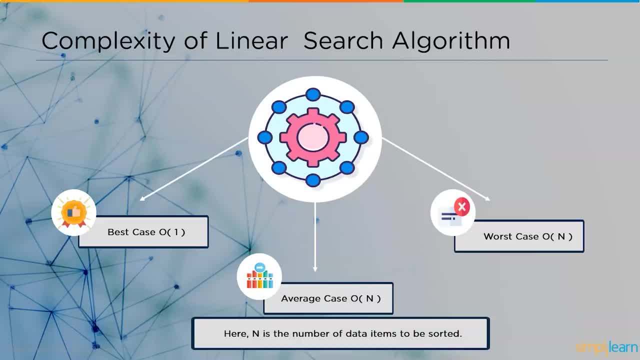 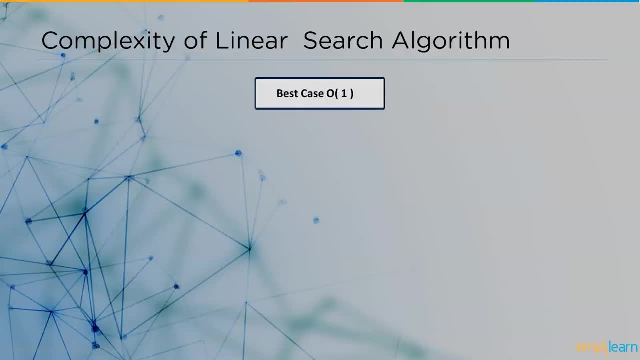 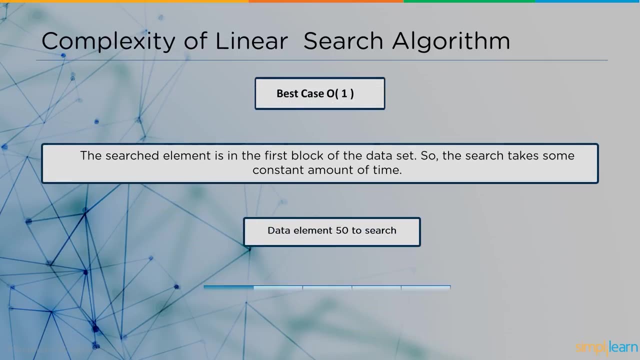 O. Here, N is the number of data items to be sorted. Let us look into how all these complexities of linear search algorithm play out in detail. First, we have the best case, which is big O. As a result, the best case scenario happens when the searched element is found in the 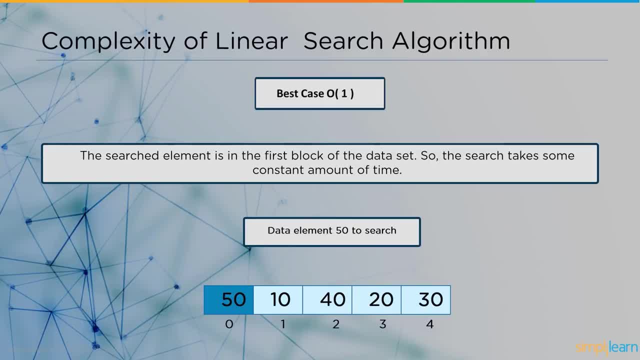 data set's first block. As a result, the searched takes a constant amount of time. Here is an example of an array with 50,, 10,, 40,, 20, 30 as the elements. Now our searched element is 50,, which is located in the first location of the array. 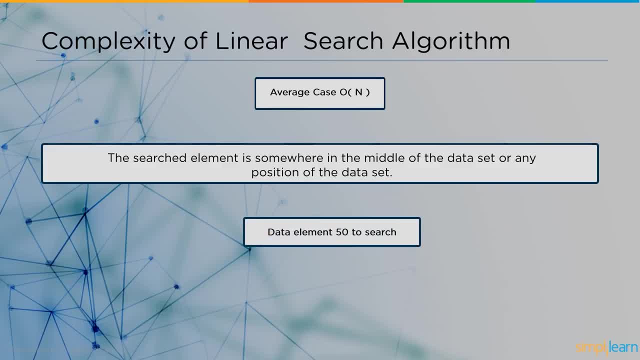 Then there's the typical case of linear search algorithm, which has big O and occurs when the searched element is in the middle of the data set or any point of the data set. the same searched element 50, we can easily see that the element 50 is present in the center of. 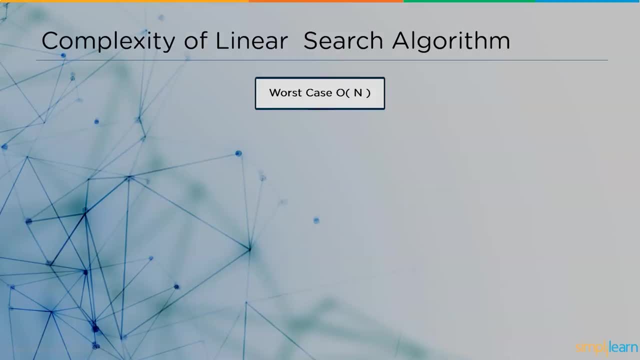 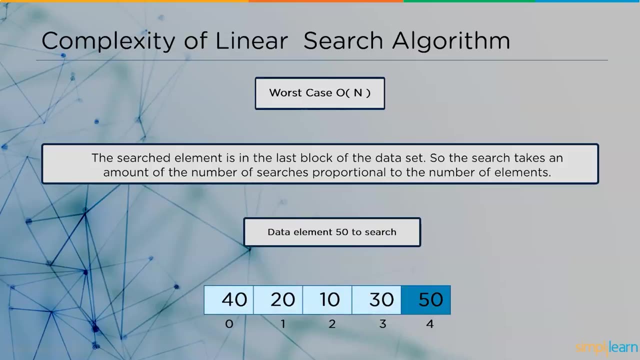 the array at the location number 2.. Finally, we have the worst case, which is O, which is same as that of the average case of the linear search algorithm and happens when the searched element is in the last block of the dataset As a result of the number of searches required. 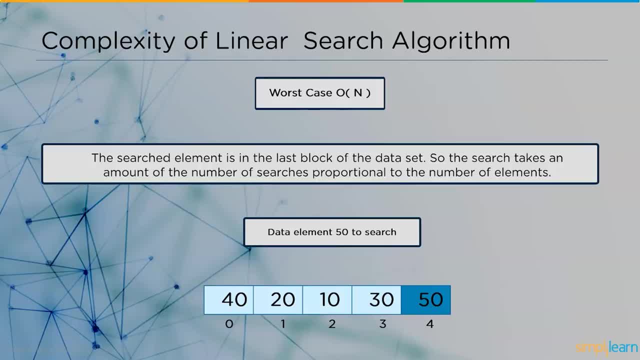 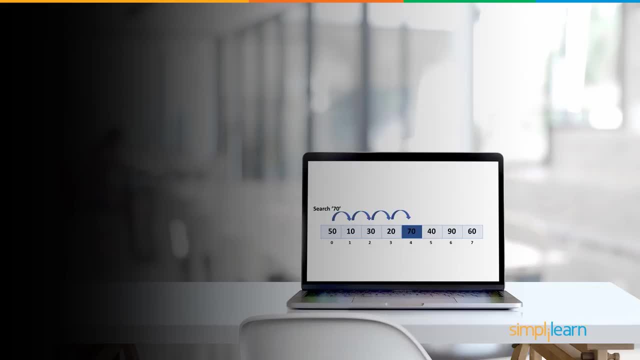 is proportional to the number of elements. as demonstrated in this example, the searched element 50 is found in the last block of the array index, which is 4.. In the next segment we will look into some real-world instances of linear search algorithms. According to the first application, 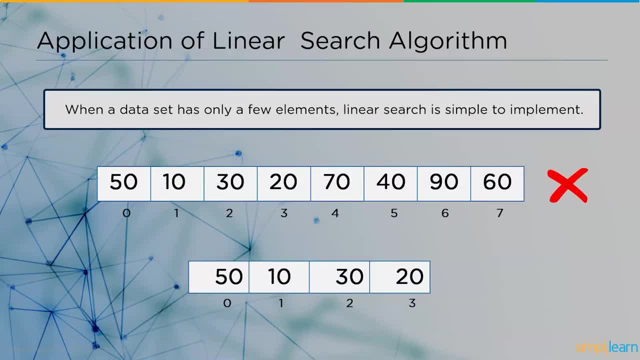 of the linear search algorithm. linear search is particularly efficient when it comes to discovering a particular string. Next, we will look into the second application of linear search algorithm. When a data set has only few elements, linear search is the simplest to implement. 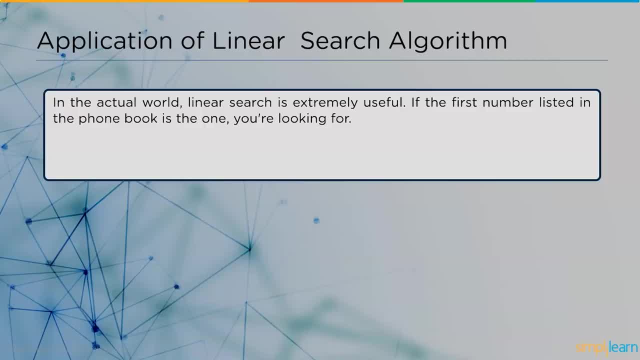 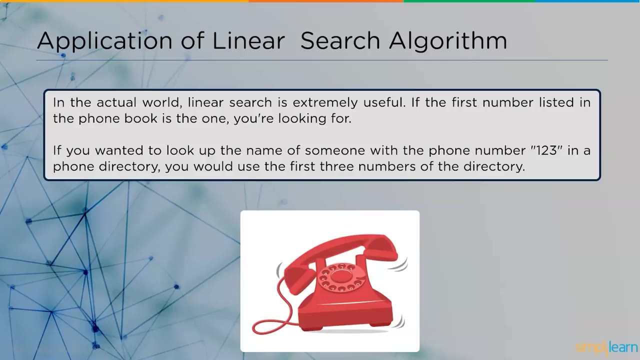 The final real-world application of the linear search algorithm is with the help of telephone directory. You may find out the name of a person with the phone number 123. This can be implemented easily using linear search algorithm. Now let us have a look at the linear search algorithm working. 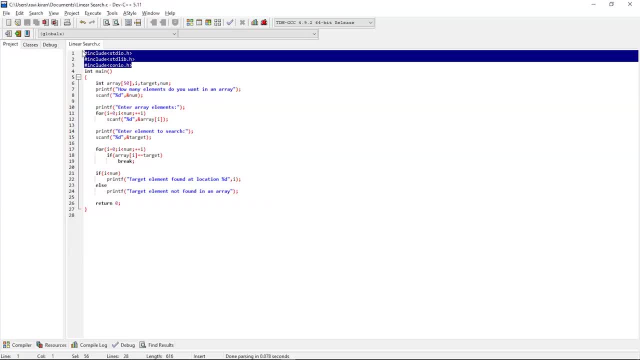 in practical demonstration. So on my screen we have an example for linear search algorithm. We have included three libraries: standard input output standard library and console input output library. Then we have entered the main function, where we have declared an array with maximum size of 50. 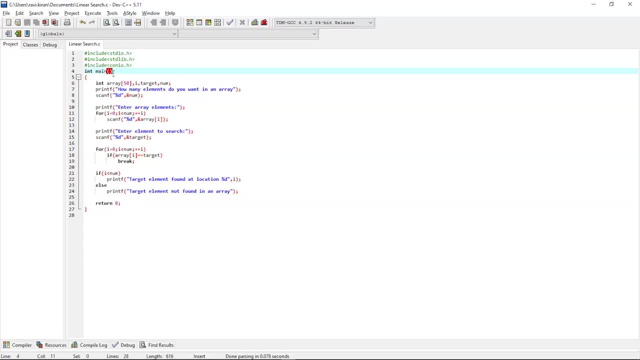 elements, a counter variable i, a variable named target, where we would store our searched element, and finally, num variable, where the number of elements in the array is recorded. Then we have a printf function to ask the user how many items are there in the array, and then we use a scanf. 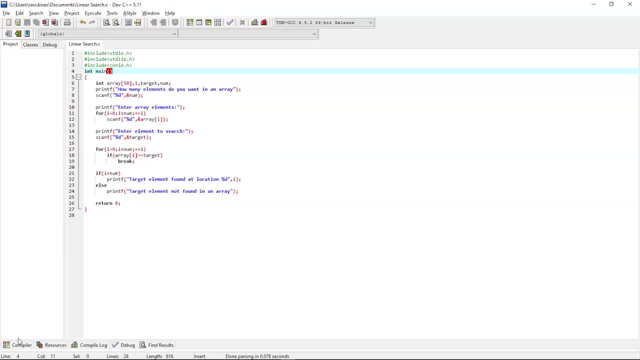 function to allow input from the keyboard. So we have added %d format specifier to the scanf function, which is used for numeric values, and num variable. Then, using a for loop, we will try to print all the items in the array, starting with zero and ending with num variable, which is the last.